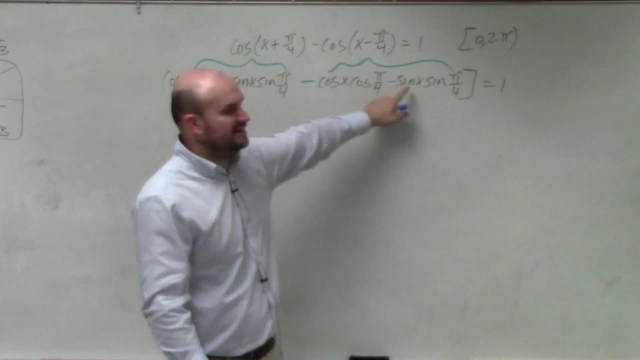 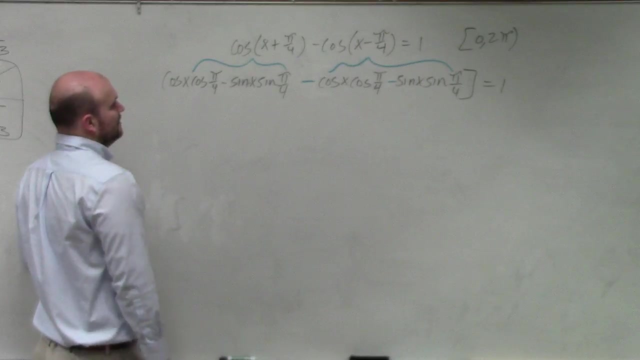 Because what does everybody do? They don't put parentheses and they just leave that negative And they leave that positive. All right, But now I need to simplify this. So, fortunately for me, I noticed that these two are exactly the same. 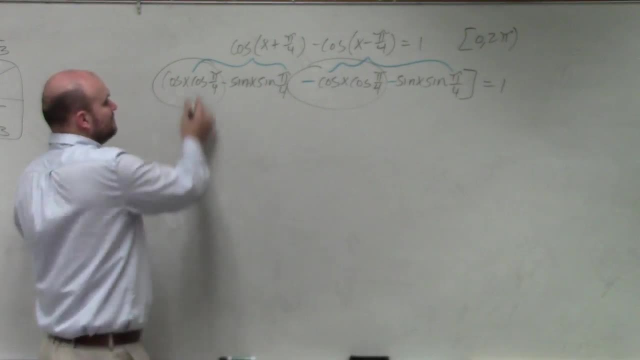 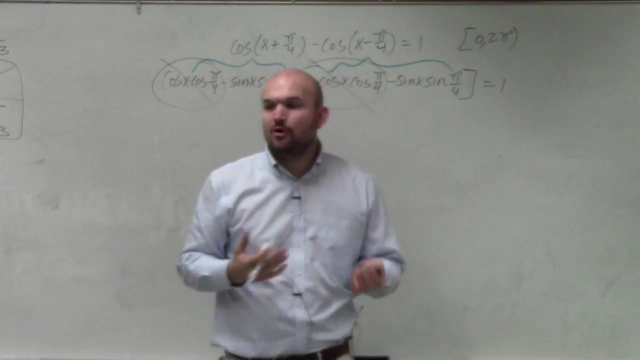 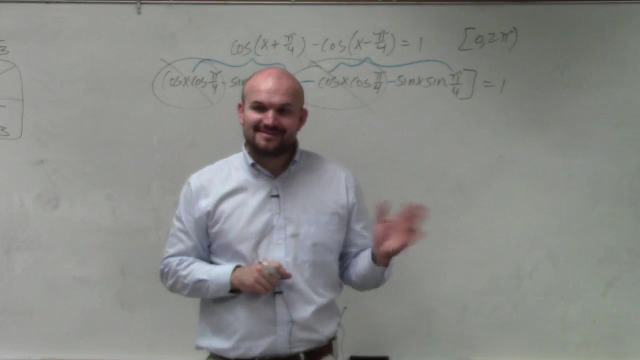 One's positive and one's negative, So therefore I can combine them to get 0.. And if you owe me $1 and then you borrow another dollar, you now owe me $2. So if you have negative x minus x, that's negative 2x. 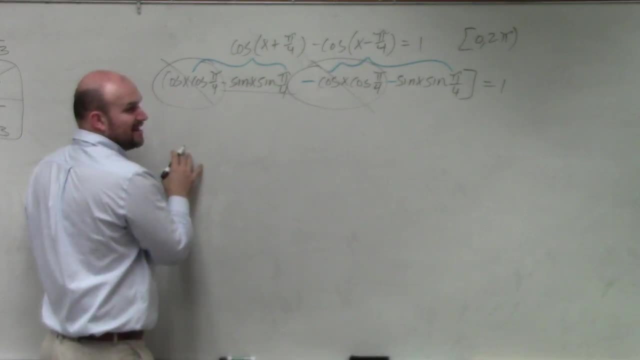 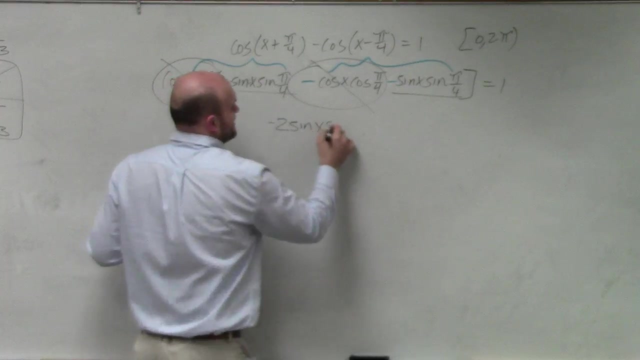 We have a negative, Negative 2x Sine x sine pi over 4 minus a negative sine x sine pi over 4.. That gives you a negative 2. Sine of x sine of pi over 4 equals 1.. 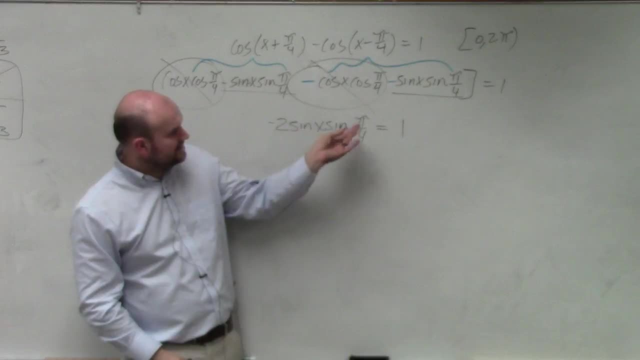 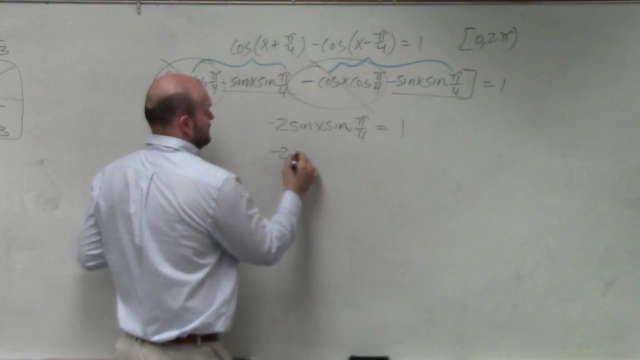 Now let's look at this: What is sine of pi over 4,, which is square root of 2 over 2?? OK, Sine of pi over 4 equals 1.. This negative 2 and 2, that divides to 1.. 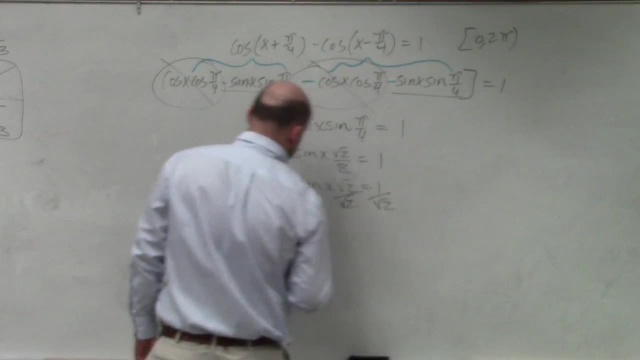 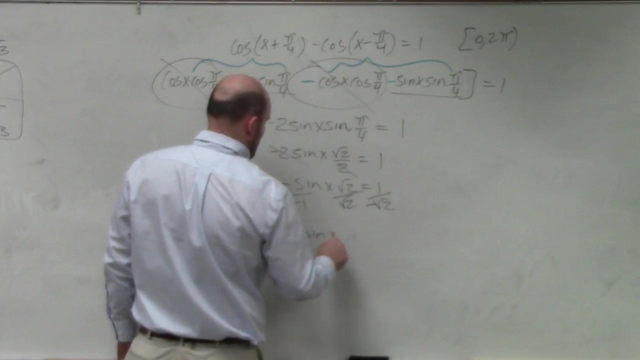 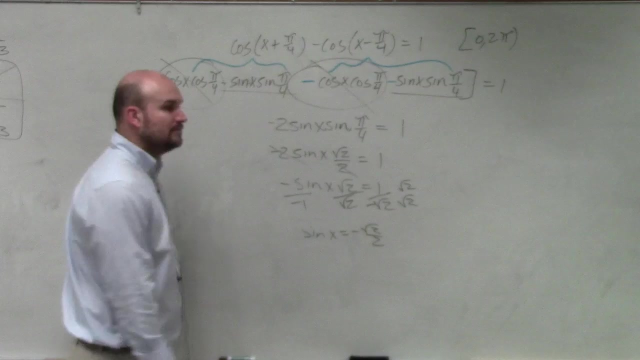 Now all I have to do is use my inverse operations. And, guys, remember, you have to rationalize the denominator. So I've solved it: Sine of x equals negative square root of 2 over 2.. But again, what are we looking for? 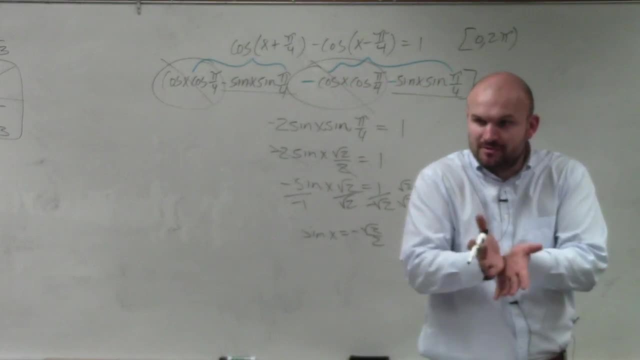 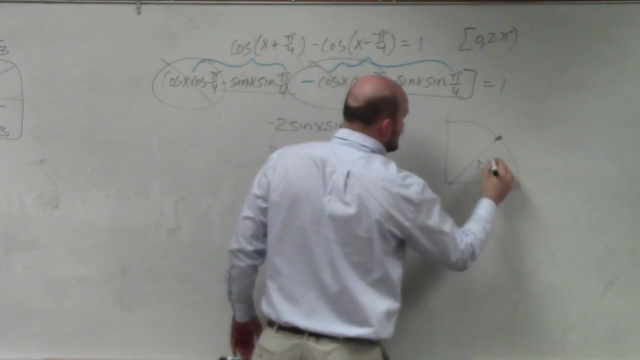 We're looking for the x. What angle gives us negative square root of 2 over 2? Within 0 to 2 pi. So we know that positive pi over 4 gives me square root of 2 over 2, comma, square root of 2 over 2.. 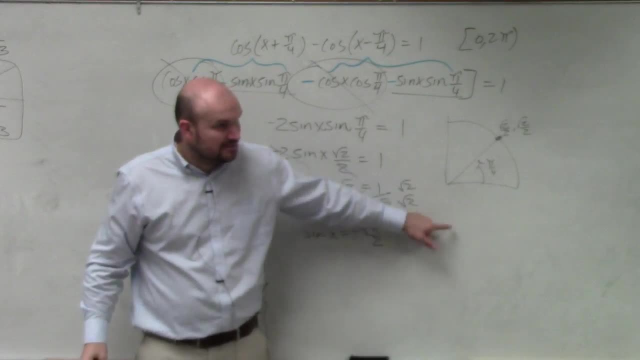 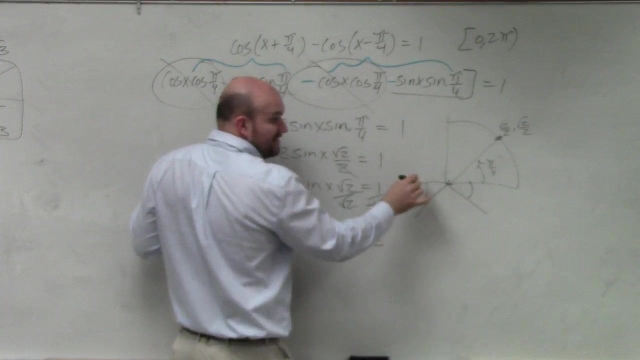 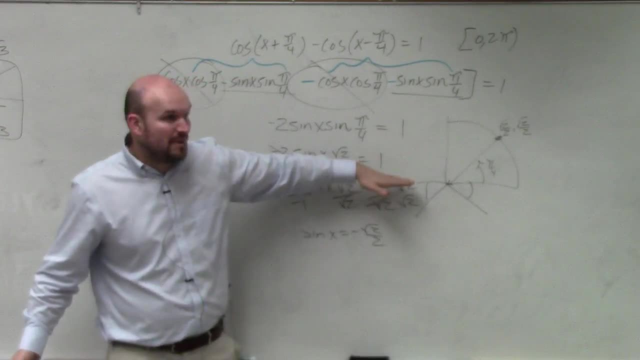 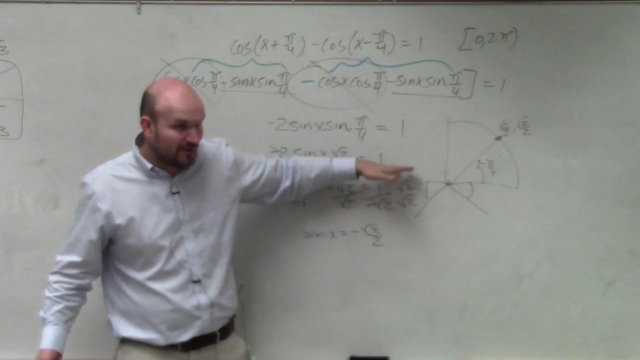 So it's halfway around the circle is 4 pi over 4.. So an extra pi over 4 would be Halfway around the circle, is 4 pi over 4.. An extra pi over 4 would be 5 pi over 4..